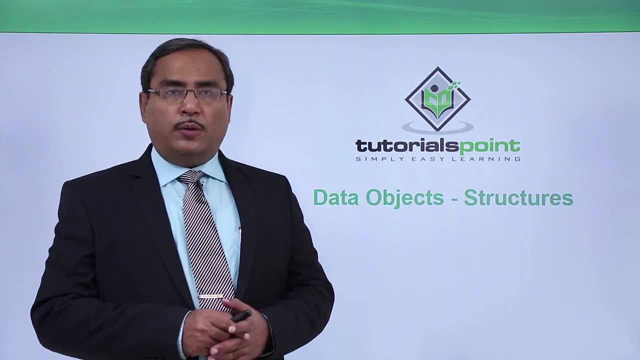 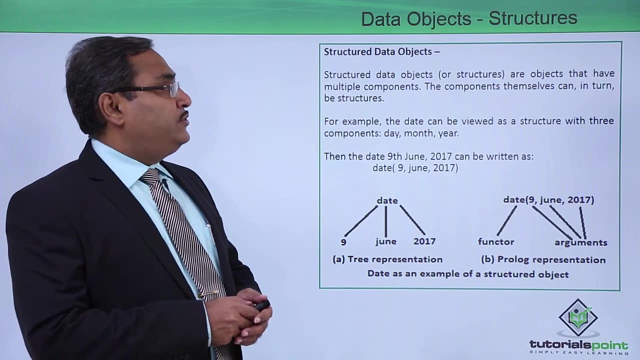 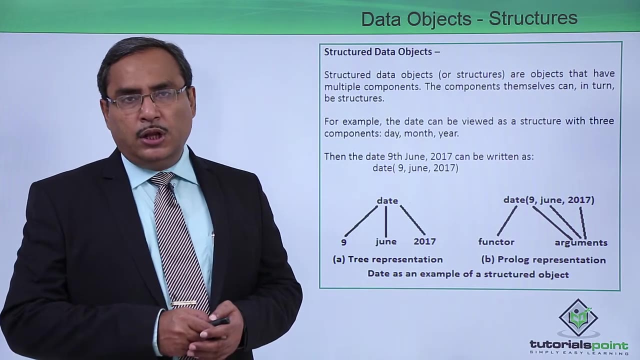 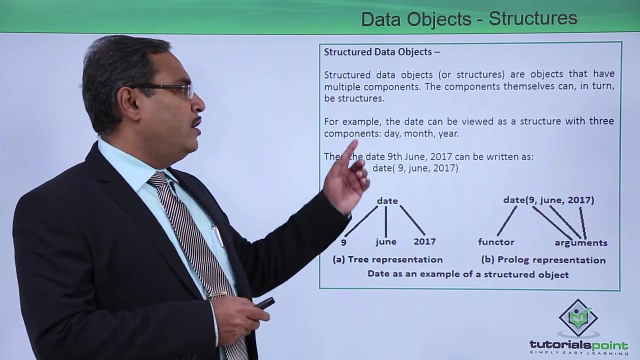 We are going to define another data objects known as the structures. So what is a structure? So here is the detailing for it: Structured data objects, or it will be called as structures, are objects that have multiple components. The components themselves can, in turn, be also another structures in this way, For 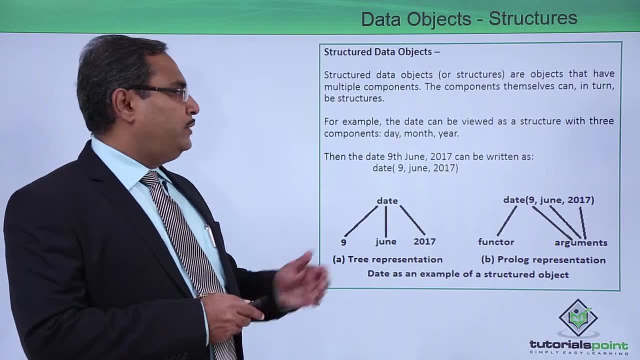 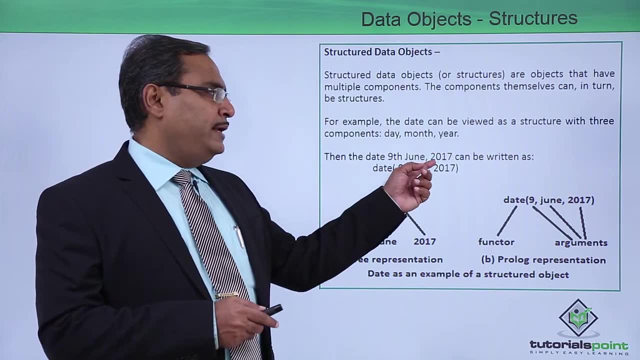 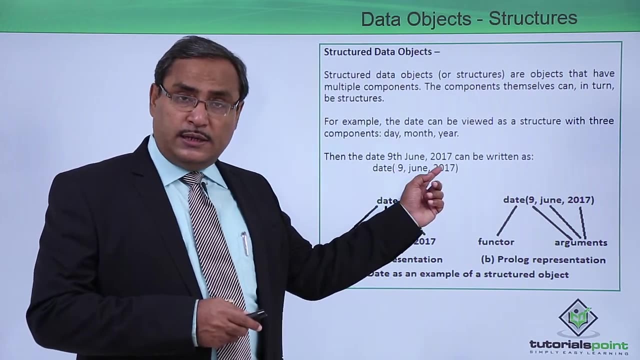 example, the date can be viewed as a structure with three components: day, month and year. Then the date 9th June 2017 can be written in this form. So here is a date, there is a structure name and it is having three arguments: Structure: 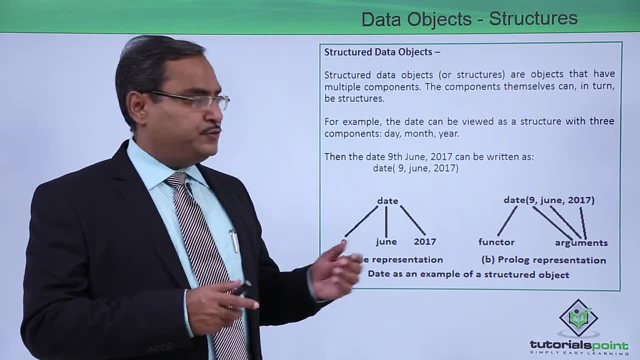 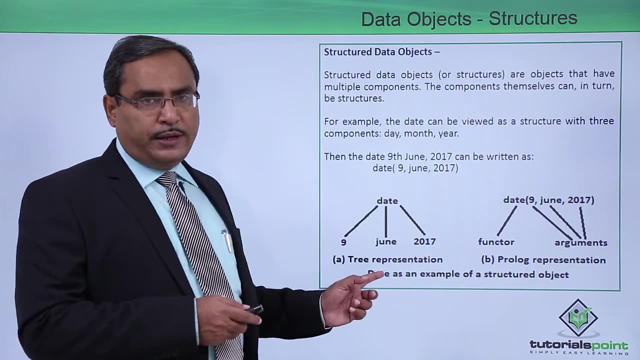 will be having multiple arguments, So that is a main feature of structure. So here we are, having this 9th June 2017.. So it can be represented in this way. All structure can be represented using tree representation. so here you have this. 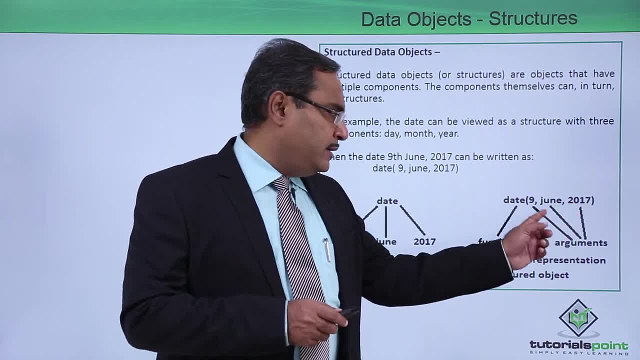 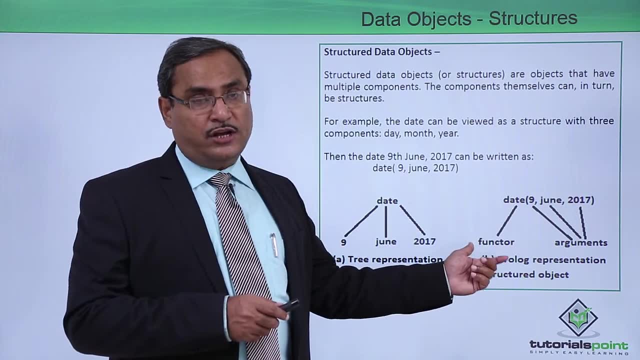 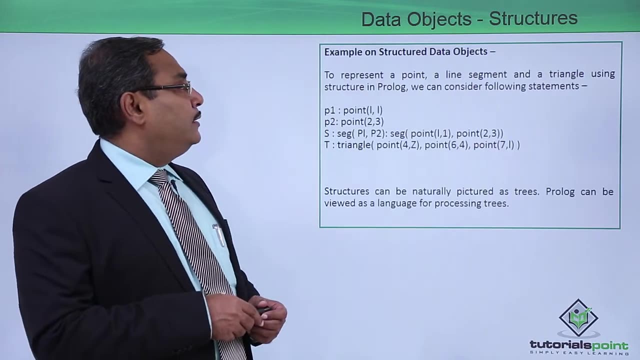 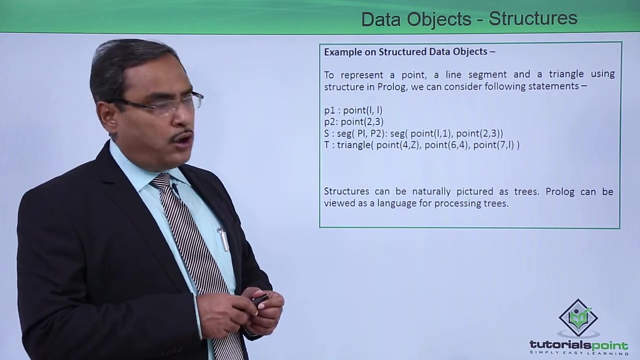 date: 9 June 2017, and these three will be known as the arguments, and this is known as the functor. that is the structure name, so please remember this term. there is a functor, so prologue representation will be like this one: to represent a point, a line, segment and a triangle using structure in prologue, we can 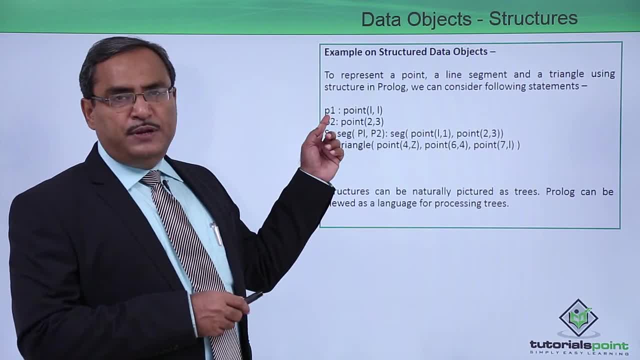 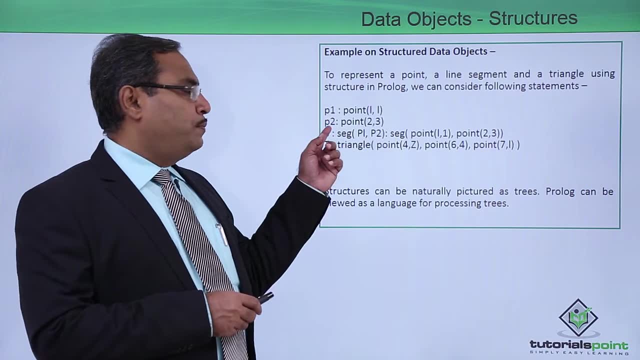 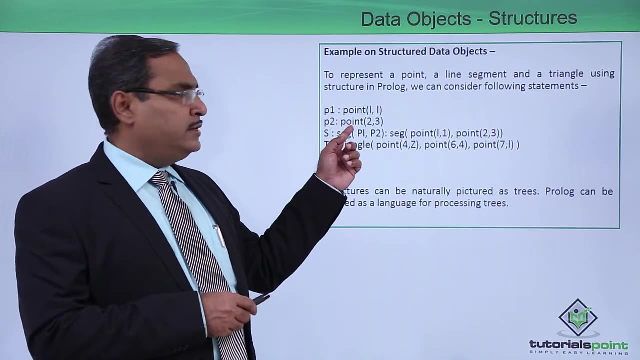 consider the following statements. so point P 1 can be represented using this functor point with X and Y as 1 comma 1. so P 2, that is a structure variable, can represent this point. that is a functor name. that is a functor rather, 2 and 3 are. 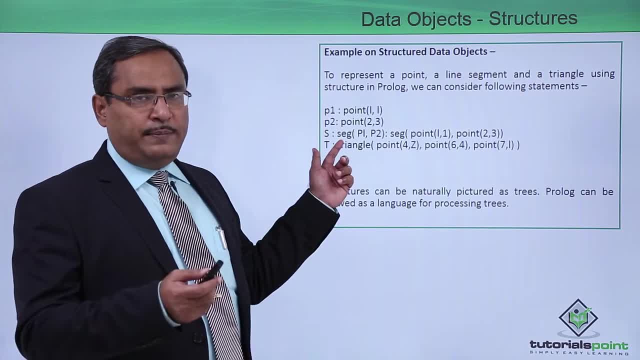 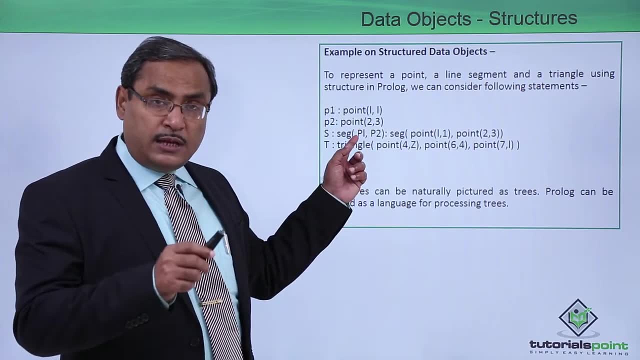 two arguments. so S segment. obviously a segment will be connecting two points and a line segment will be connecting two points and a line segment will be connecting two points and a line segment. so here we are having this: P 1 and P 2, and P 1 and P 2 they are themselves are separate structures. so point 1, comma 1. 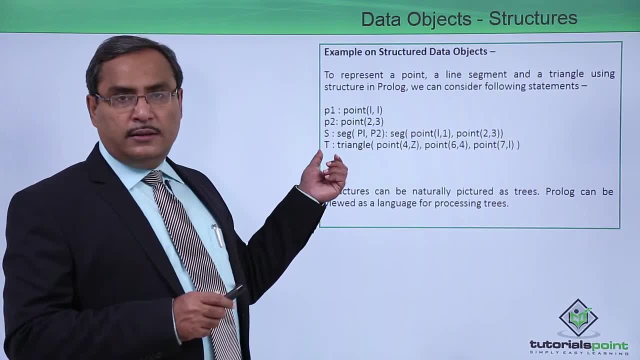 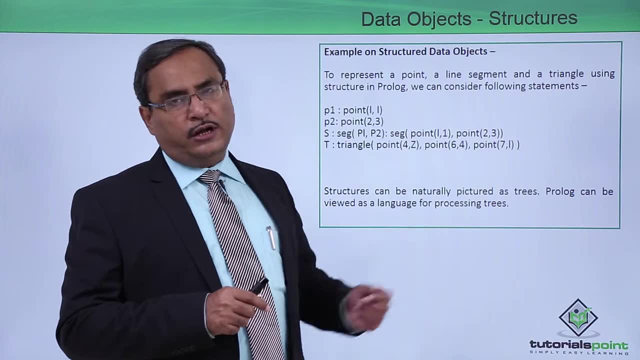 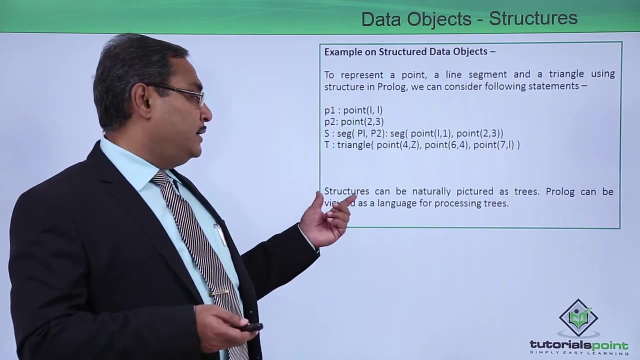 and point 2 comma 3. so triangle will be having three points at its corners. so triangle can be represented using these structures. so here we have used the variable name also. that is also allowed. otherwise I can put some number there. structures can be naturally pictured as trees.